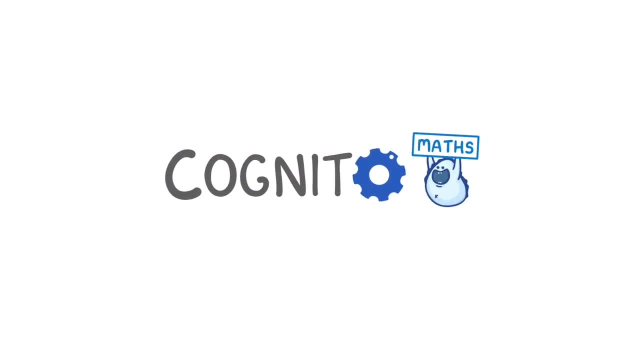 In this video we're going to cover 2D projections of 3D objects, which just means taking a 3D object like this one and considering what it would look like from different views or perspectives. The three 2D projections that you need to understand are the front elevation. 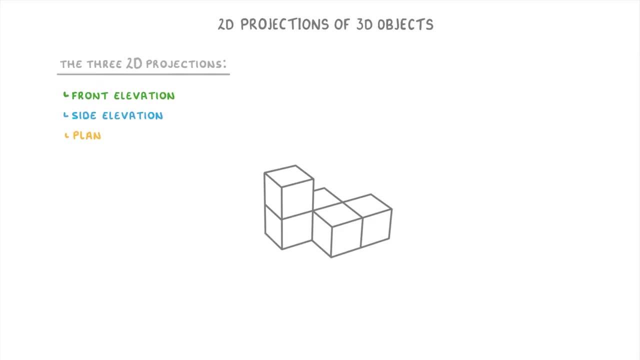 the side elevation and the plan. The front elevation is just what the object would look like if you were looking at it from the front. So if you imagine that you were looking at it from this angle, you would only be able to see these four faces that are directly. 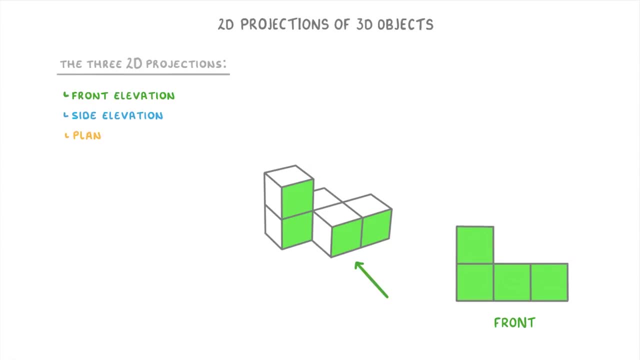 facing you, And so you'd basically just see a block like this. Meanwhile, the side elevation is the same idea, but this time it's the view you'd have by looking at it from the side over here. So this time you'd just see these three squares, And so it would look. 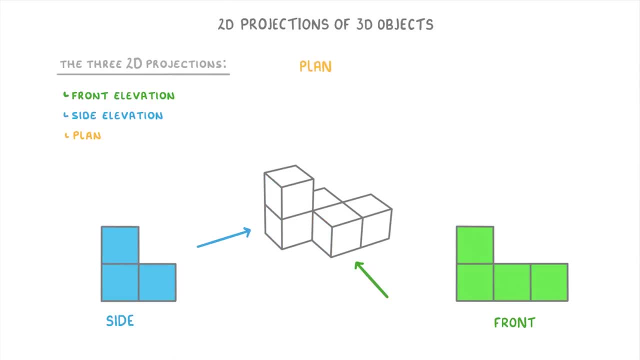 like this. The last view is the plan, which is a bit different, because this time it's as though you're taking a bird's eye view, looking at it from above, So you're only going to see the squares facing directly upwards, which would be these four squares. So it would 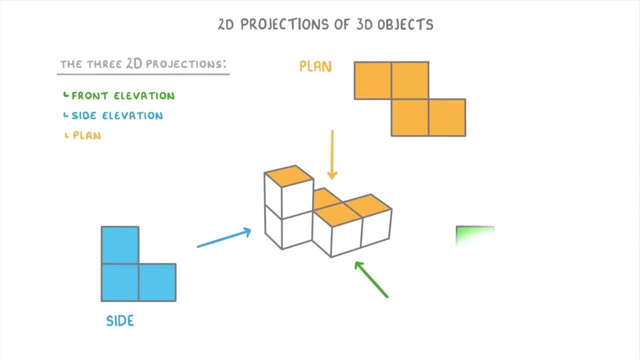 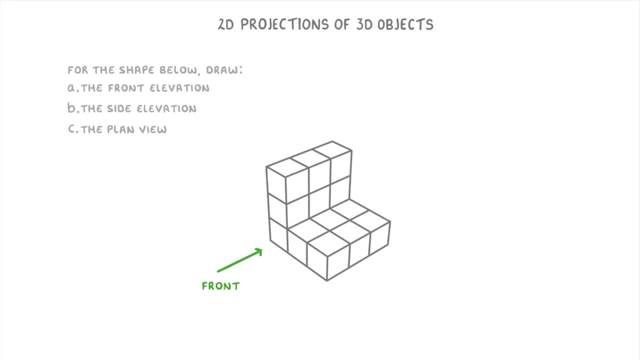 look like this. Let's have a go at another one and feel free to leave a comment if you have a question. So for this question you need to do basically the same thing: You need to draw out the front elevation, the side elevation and the plan view of this shape that they've given us. 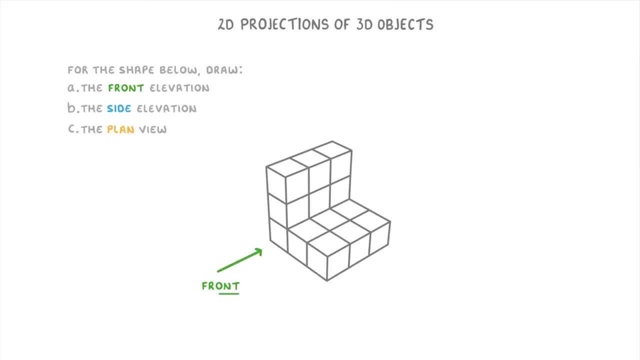 Notice, though, that this time, the front view is labeled as this side, And they'll always do this in the exam, so that you know which side is which. We can then figure out that this side must be the side view and, as always, this view. 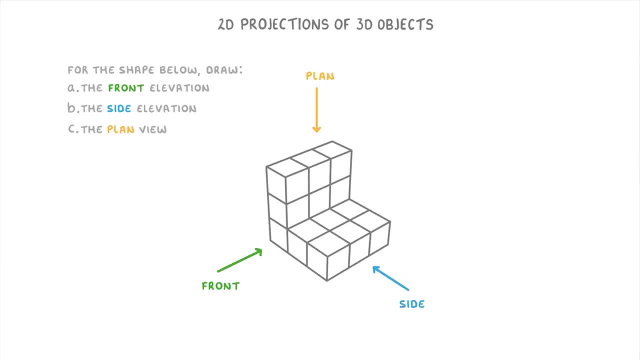 from above will be the plan. So, from the front, you'll see these five squares, which will give us a 2D projection like this. Meanwhile, from the side, you'll be able to see all of these nine squares, and so the